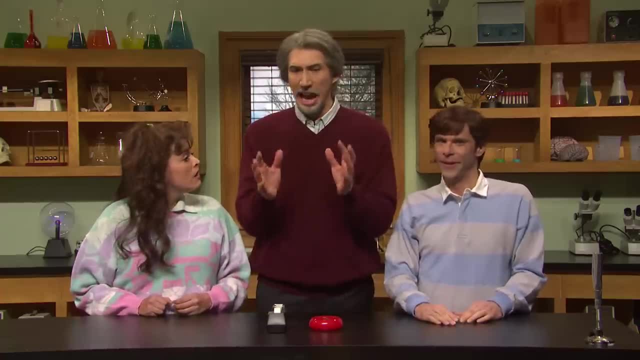 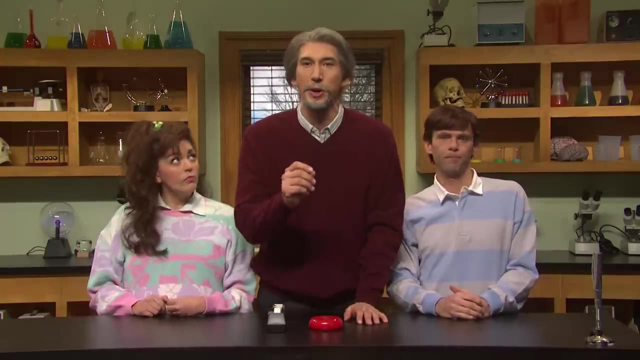 Imagine you're in a pool. Mark out Guys, Hold up. Guys, Fish out of water. Stop, Forget about that. Forget about the pool. No more pool, Let's just do the experiment. And for those of you, doing the experiment along with us at home: 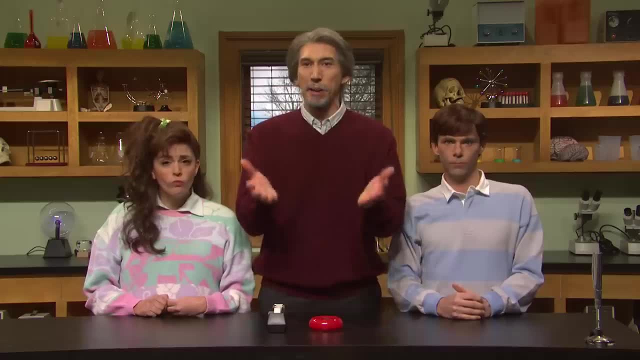 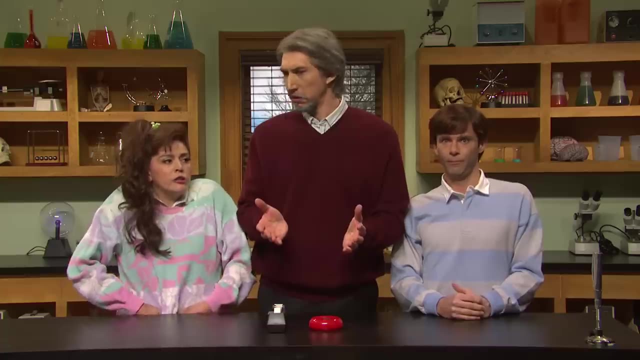 make sure a parent or guardian is present, because what comes first in the science room? Um, the guy, The guy, Yeah, my older sister said the guy like always comes first. I don't know what that means. Oh my God. 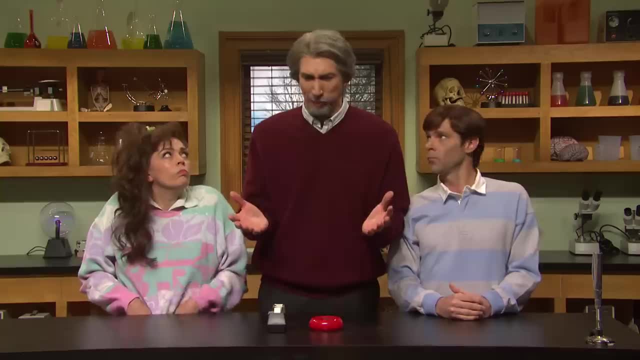 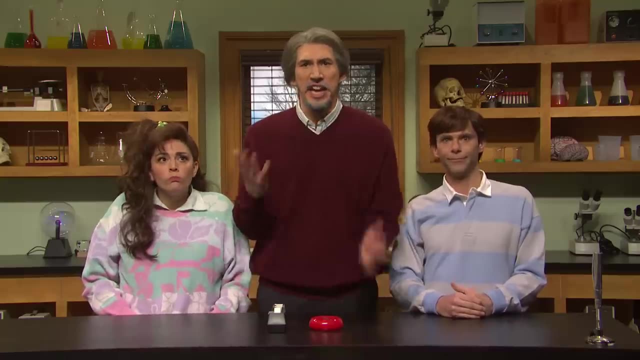 No, no, That's not what that means. The guy does not come first here, The girl comes first. No, my sister said the girl never comes first, It's safety. Safety comes first. That was an awful conversation we just had. 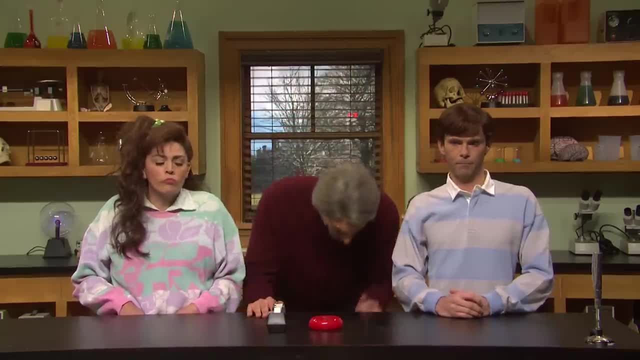 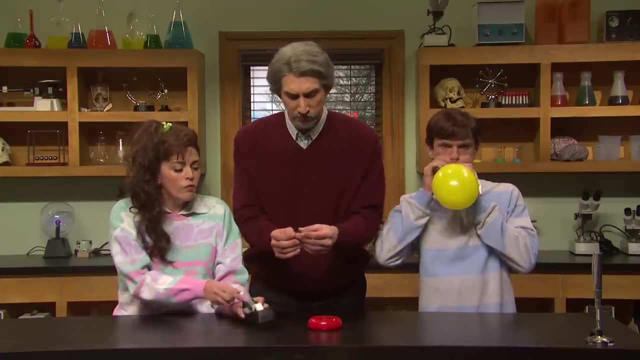 Now for today's experiment. we'll need a balloon. Josh, why don't you blow one up? We'll also need a sewing needle and some scotch tape. Oh my God, Josh, you passed out. Are you all right? 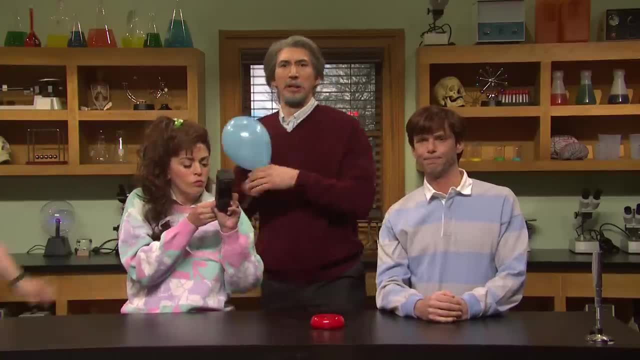 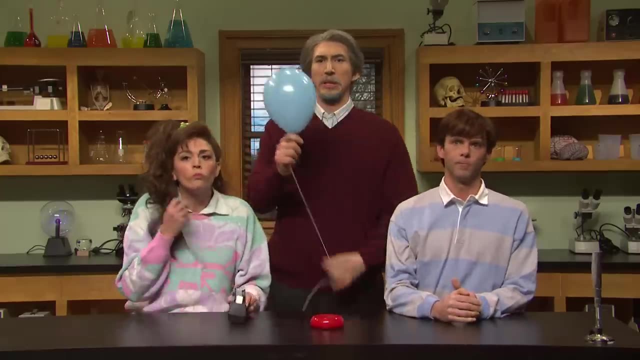 No, Yeah, What? All right, Can I get another balloon? Okay, guys, back Now. look at this balloon. No, back up, Back back, Just a little way over. Now we're going to put a piece of scotch tape on it. 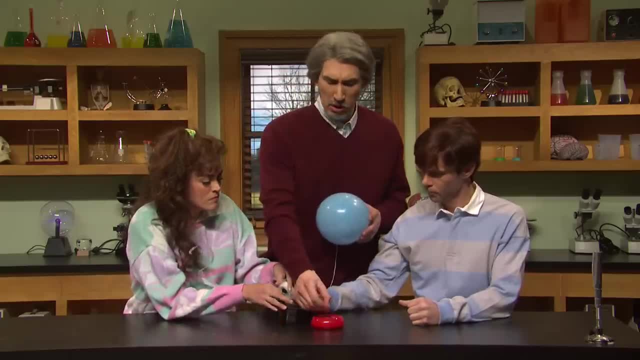 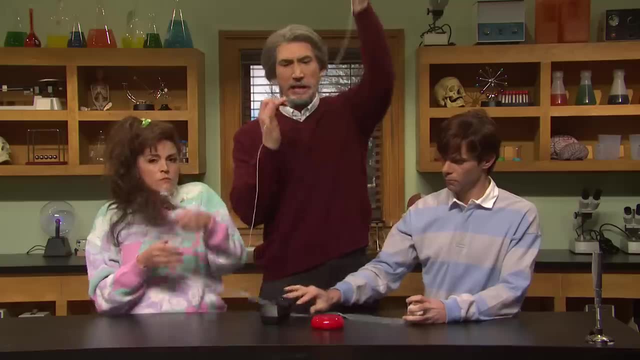 and see what happens if I put something sharp through the scotch tape when I: Okay, stop messing with this, Put this down. What will happen if I put a needle through the scotch tape through the balloon? Um, it'll get vaccinated. 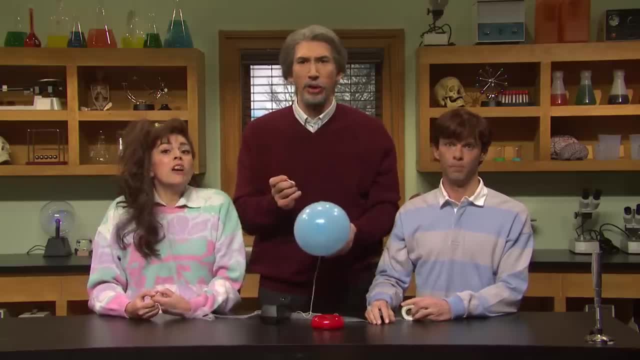 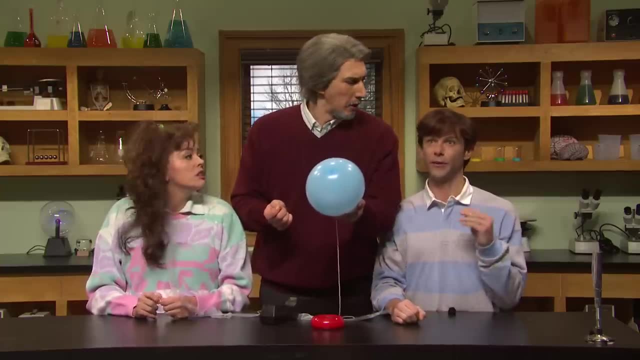 What? What would normally happen? if I stick a needle through the balloon, It'll scream: Look you stupid, stupid kids. What do balloons do? Um, provide a sense of atmosphere. If I stick a needle through an effing balloon, it will. 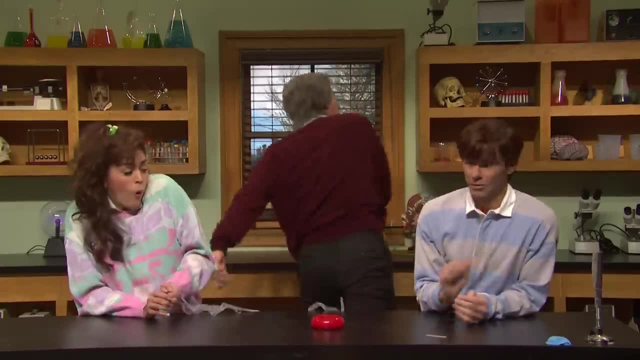 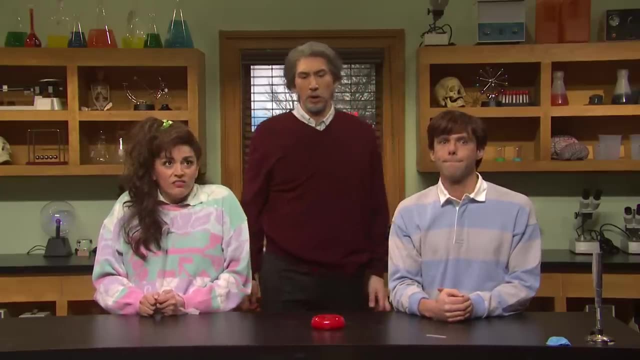 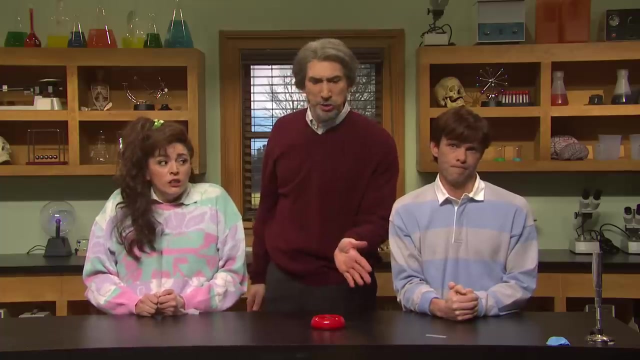 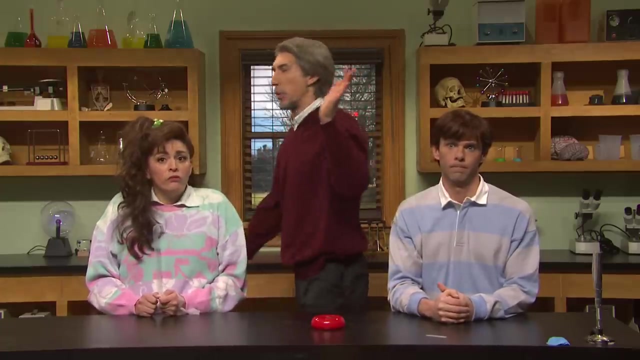 What Come first? Oh, If punctured balloons will. Starts with a P, ends with a bop, It'll bop, Yeah, bop. All right, go to that video with the ducks flying, because I'm about to scream the C word into my shirt in three, two, one. 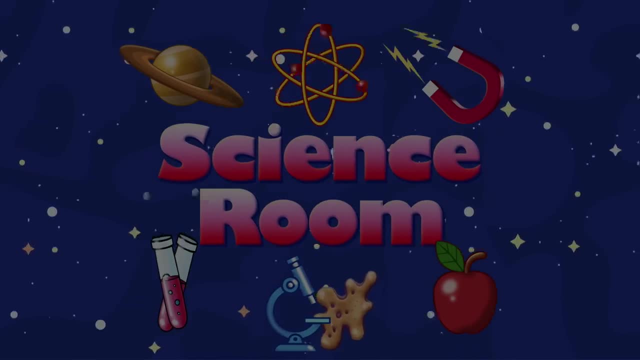